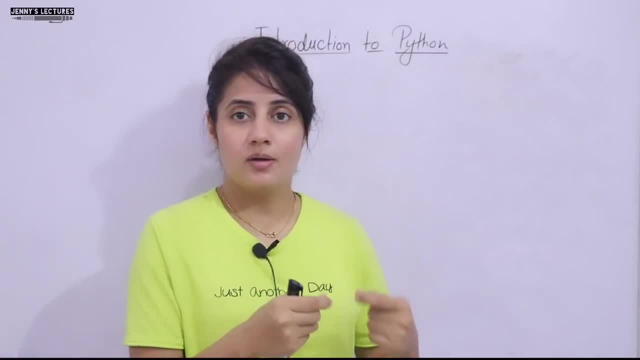 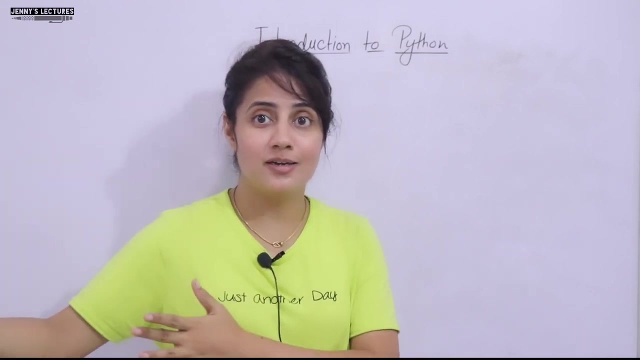 have noticed. if you suppose, Nowadays I you know I search for specially chicken curry kurta Right. So I have. I have been looking for these kurta's in two or three website shopping websites and whenever I open any other website, you know, for study that kind of thing. So those relevant. 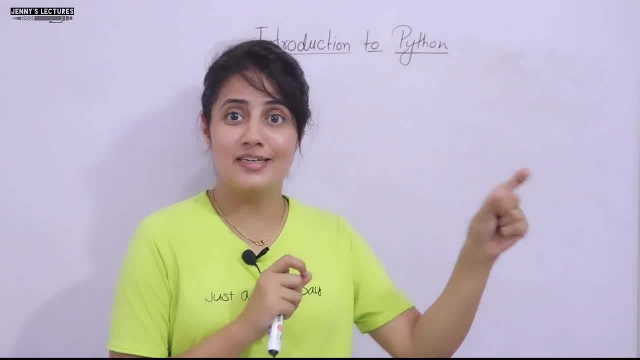 ads. they show me now ads of those chicken curry, kurta's and all. So whenever I open any other website, you know, for study, that kind of thing, So those relevant ads, they show me now ads of those and all. so how they come to know the advertisers, like how they come to know that I am interested. 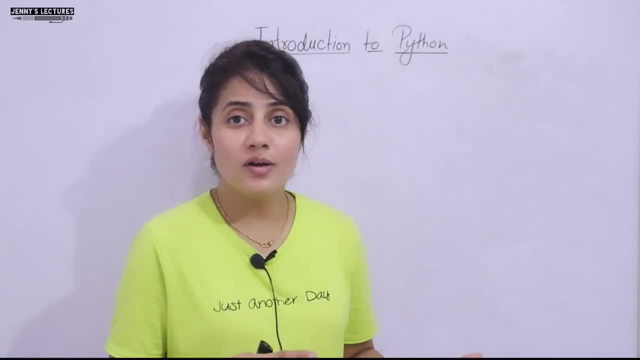 in buying those chicken curry kurtas. so this is what they have: analyzed my data. how many websites I have visited in which how I am interested. so they have analyzed that data. they have collected my data. they have analyzed that data and according to that they have. 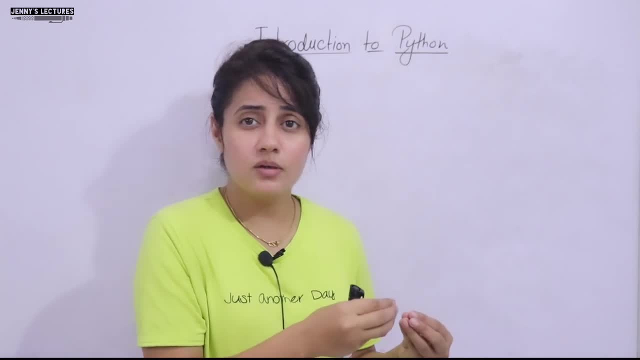 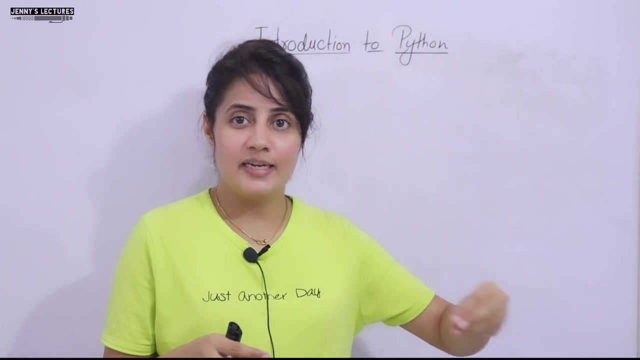 mined. you can say some pattern they have formed and they come to know that I am interested in chicken curry kurta, so they show me the relevant ad. I think you must have noticed this thing also, right? so this task is what, this analysis of data and all in this also. 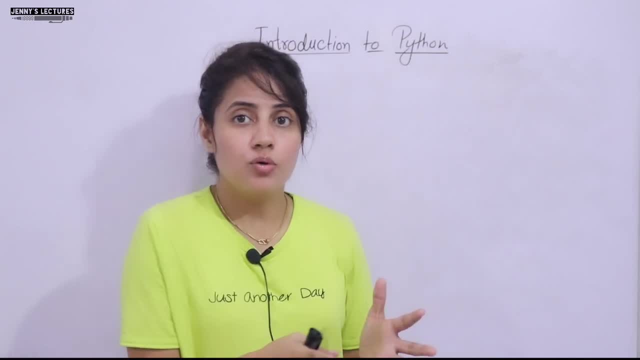 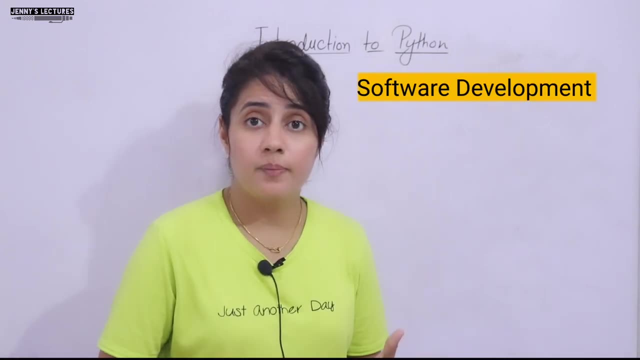 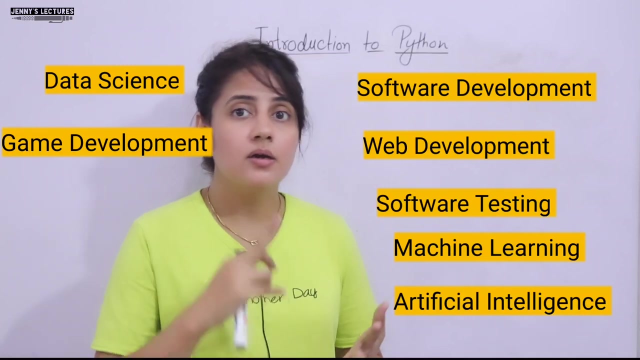 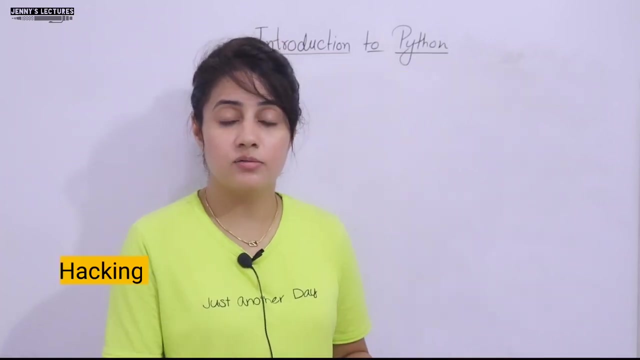 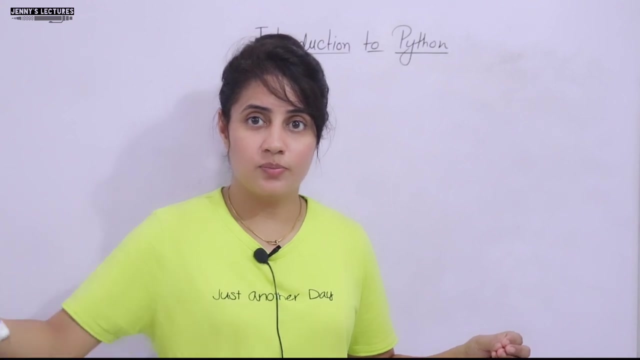 python is being used right. so in many areas this is one application of this language. and see, in many areas like whether it's software development, it's web development, software testing, machine learning, artificial intelligence, data science and so on and so forth and so on and so forth, and finally, this is not been used in like the psychology and security. 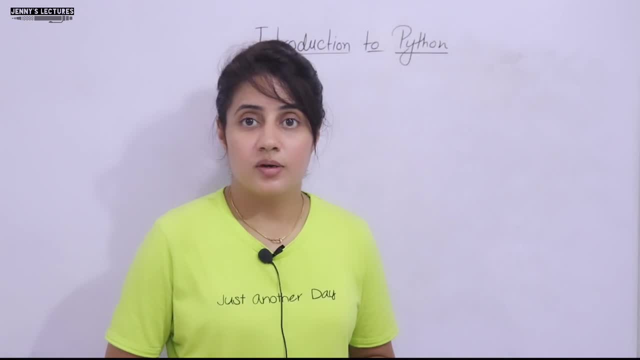 regions and this is wrong. data science, game development, making of any apps, mobile apps. these big giants are using this language right And the person who are using it- researchers, scientists, software developers, software engineers, software testers, game developers, mainly data analysts and even school going kids. 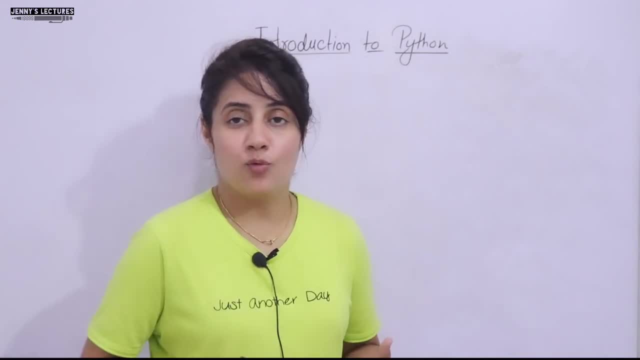 they are also learning. or you can say: using this language, See, because no researchers and scientists, they want us right, They don't want to utilize. or you can say: waste their time by learning a complicated language and Python is easy language. 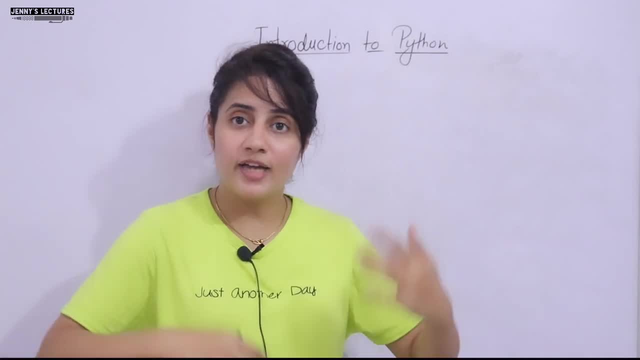 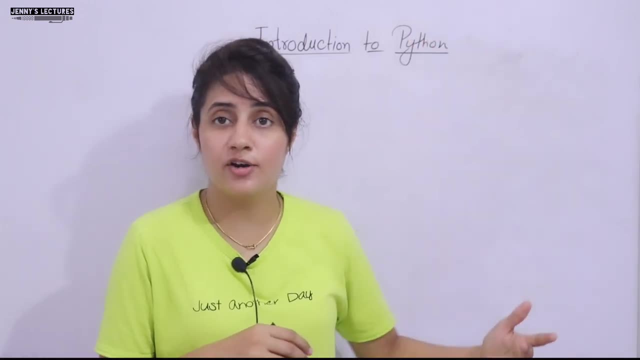 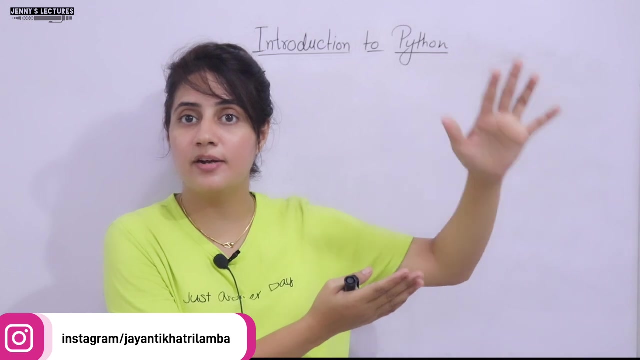 So they went for this language, Python language. So that is why recently this field is on boom: machine learning, artificial intelligence, data science, this kind of thing. So that is why, with that field, Python came into picture, because these kind of people- researchers, scientists- 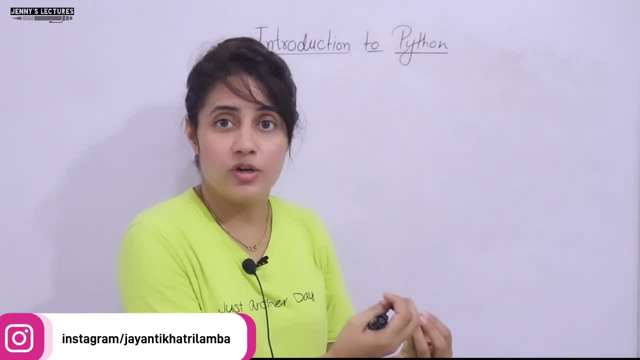 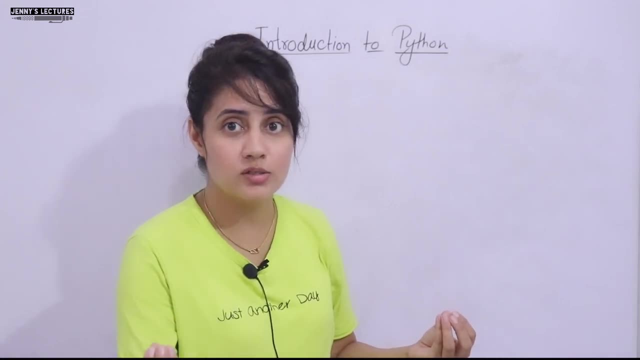 so they are working in this field. they want a simple language to work on right. They don't want to waste their time on learning a complicated type of language. Python is very simple, very easy to understand language, So they adopted for this language. 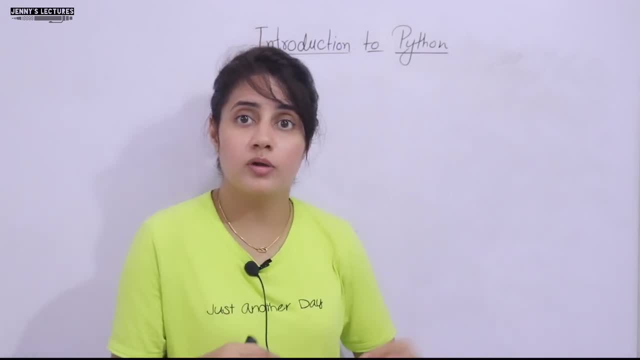 and that is why this language has become so much popular in the recent years. So why it has become so popular? Because, first thing is it is easy to learn, easy to understand and it has wide range of applications. I have told you in how many areas. 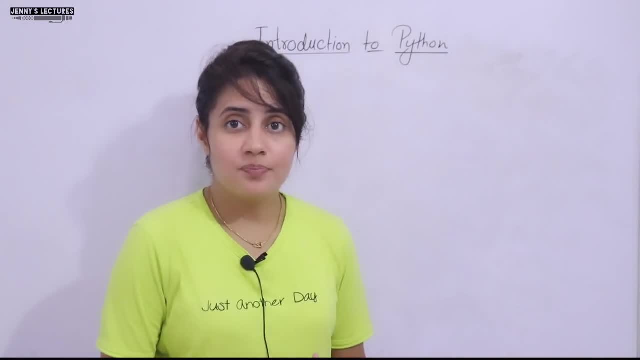 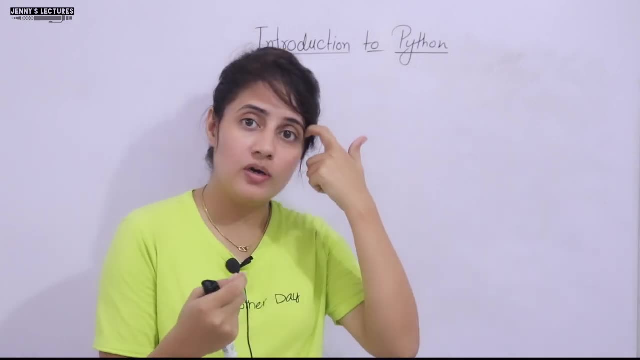 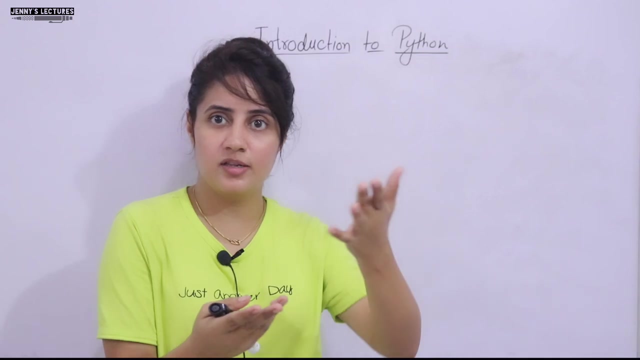 almost in every area it's been used. Second thing: you can write down. you can solve any problem with fewer lines of code. Suppose you want to print hello world in C language, So those header files, main function and printf hello world in C++- also header files. 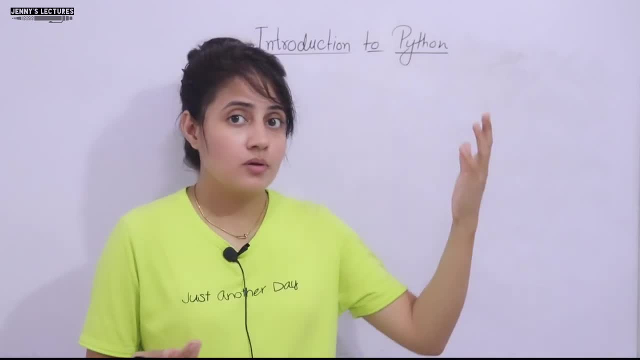 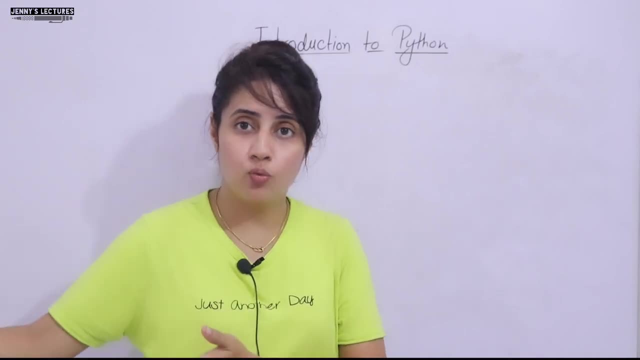 std namespace, std main function and all In Java those you can say domain function, system, sorry, public, static void main, then systemoutprintl and then hello world. this kind of thing In Python, simply what you need to write: print. 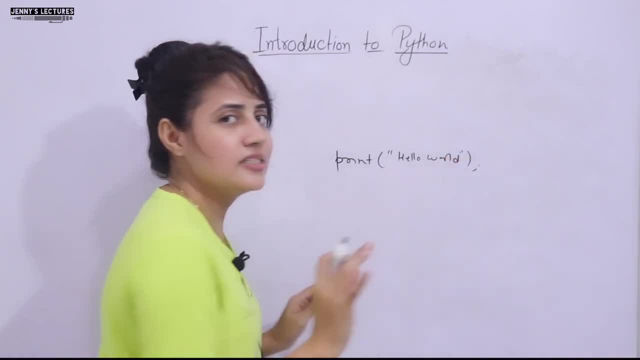 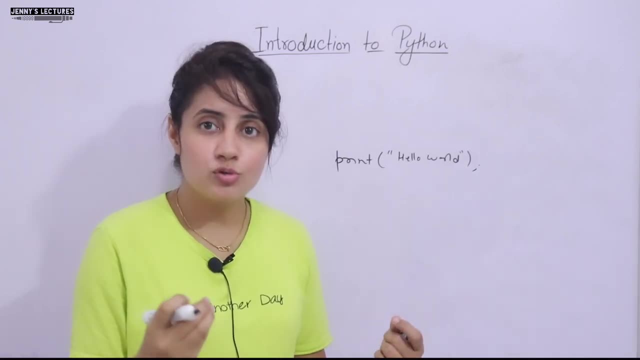 hello world. that's it, nothing else. a simple line, Nothing else. So in fewer lines of code you can solve complex problems Right And more easily you can understand the code. So it will save your time. also another benefit. 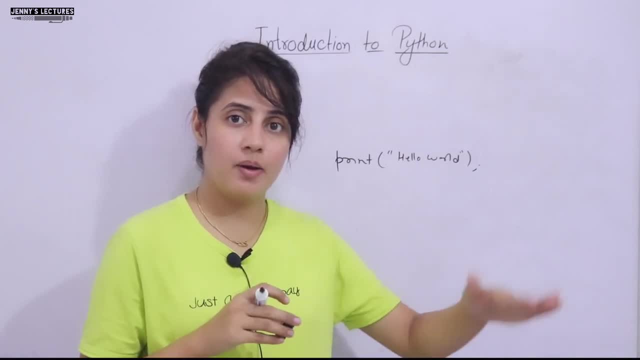 And it is high level language. You don't need to be aware about those memory management type of thing like in C. You have to aware, you have to keep track of, you have to manage your code. You can manage the memory manually. 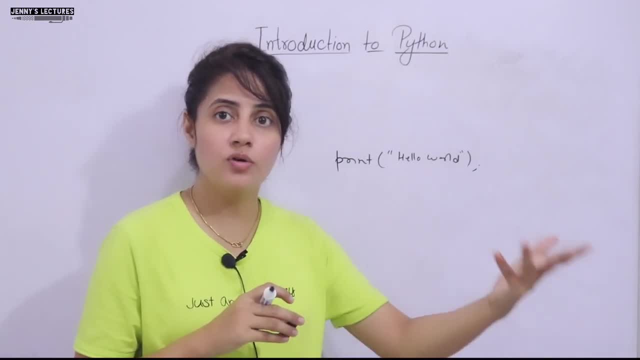 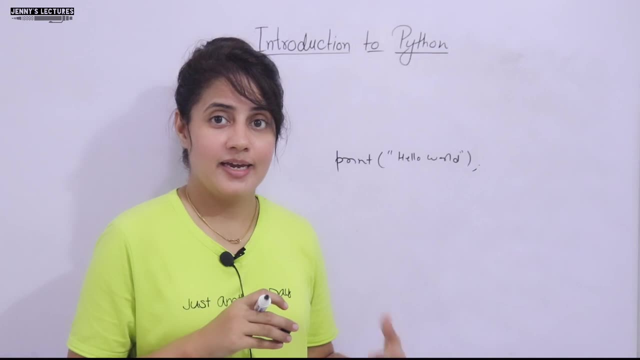 But here automatic memory management is there. It is high level language So you can do more with less right With the writing you can say less code. you can do more in this. It is object oriented programming language, but it's not like that it doesn't support. 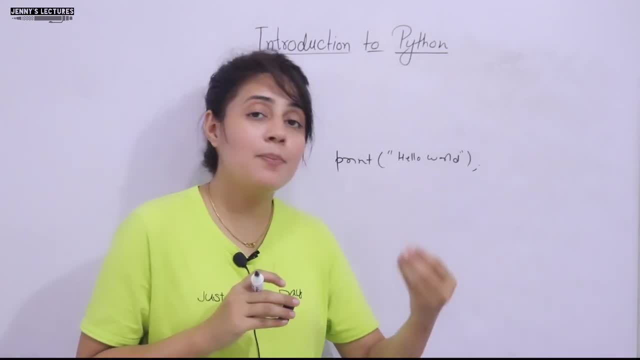 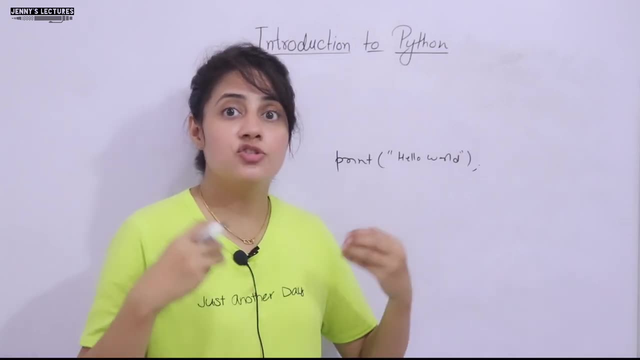 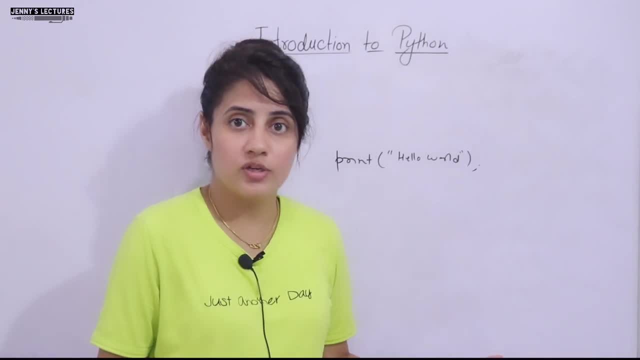 everything you can use this language, Or you can say it's multi-purpose language. It is interpreted language. These are some features of Python. You can just note down these features. So it is also Python is Python is interpreted language. 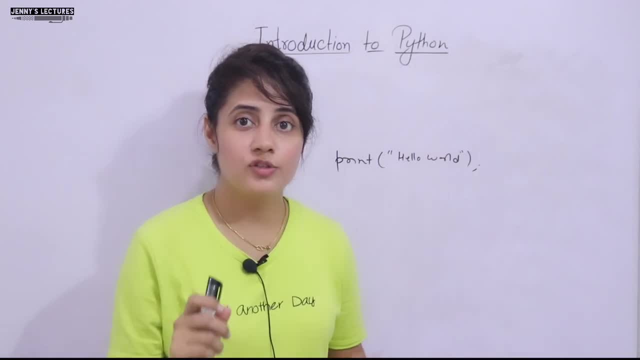 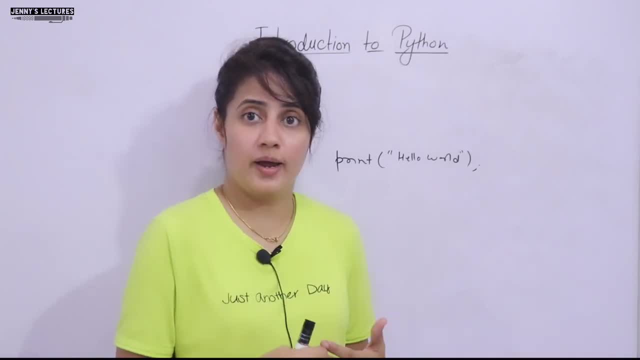 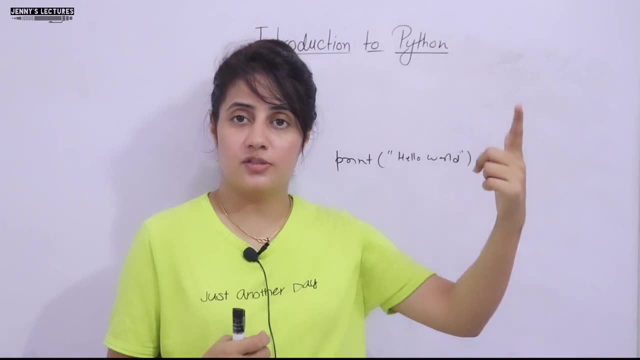 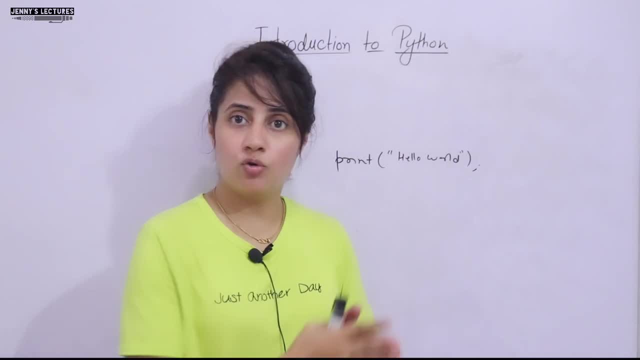 Right. They can write down their packages or functions or modules and they can contribute. It is open source. Anyone can use those inbuilt functions, libraries and all Right, Like in C and C++ also, we have some libraries in there. Redefined functions are there. 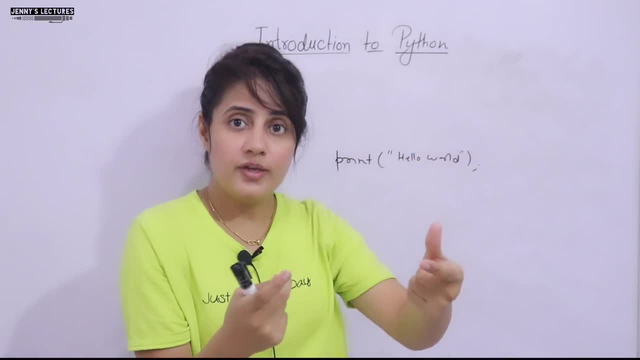 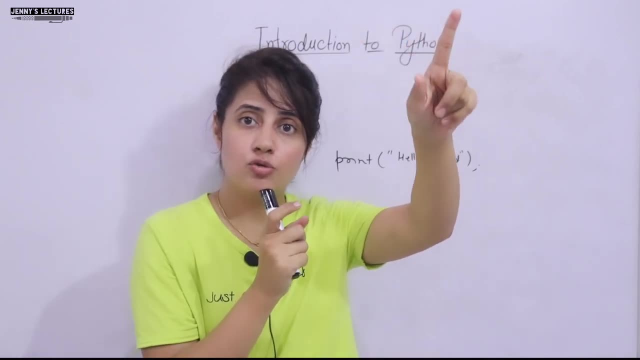 These are already defined function, Like if for string concatenation. like if for string concatenation, like if for string concatenation, we use directly a function, strcat. So the definition of that function is already in those libraries. You don't have to write down the definition of that function. 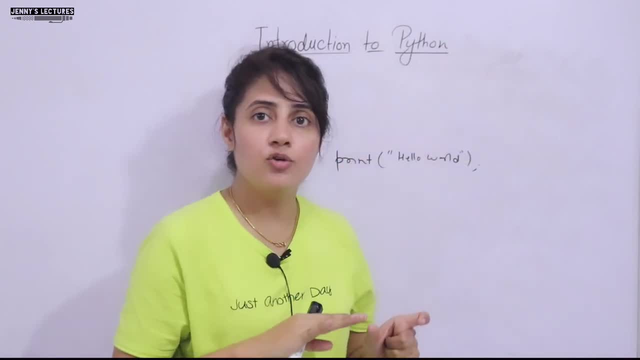 You don't have to tell the compiler. You just use that header file, stringh, and you can call that function Because it has already been defined in the library by some other people, by someone else. So same it is also having rich library. 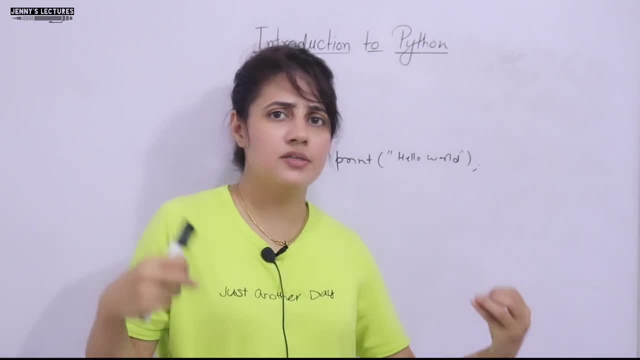 because it is open source So and huge community it is having, If you are finding any difficulty in this. so there are many forums, discussion forums- you can post your queries and definitely you will get answer. For example, some libraries are 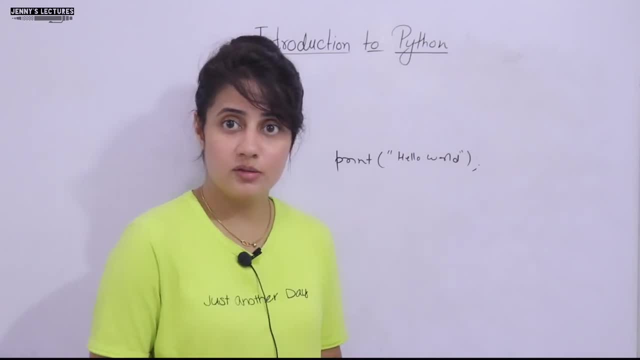 you can say NumPy Pandas, TensorFlow for machine learning and data science, while in this field they use that library. See, basically libraries are what Some codes are written, Codes of some basic functions are written on those libraries so that programmers don't have to write down those functions. 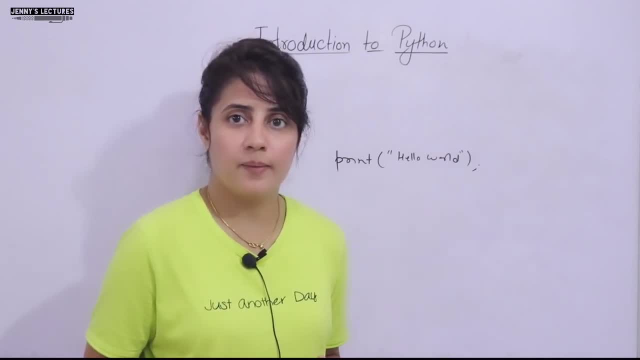 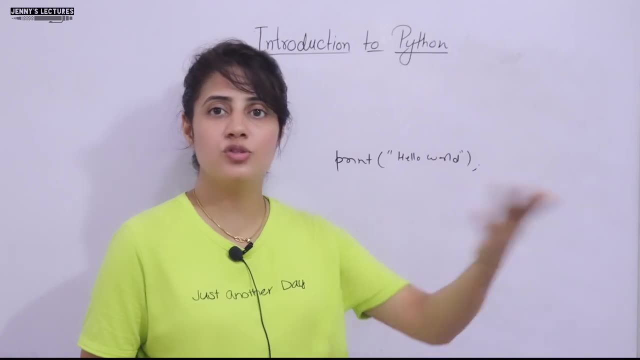 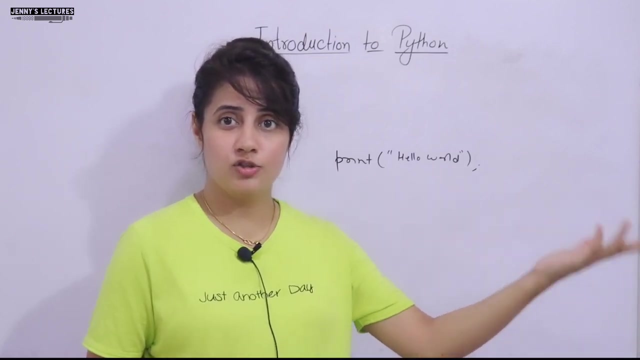 from scratch and they can reuse those functions in their own program Right, So that obviously it will save time of any programmer Right, Because they are reusing that function, Like for making chapatis, you need atta Right, So just go to any shop. 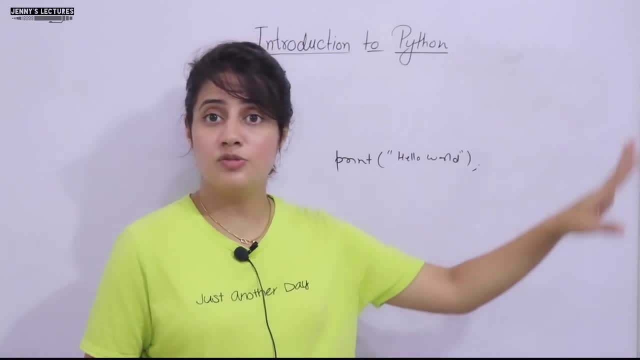 Maybe you can buy whole wheat or atta, Right. But the process behind that thing- generally farmers do that process, that long process, Right, They have done for you, So they have built those things for you. You just have to go and buy. 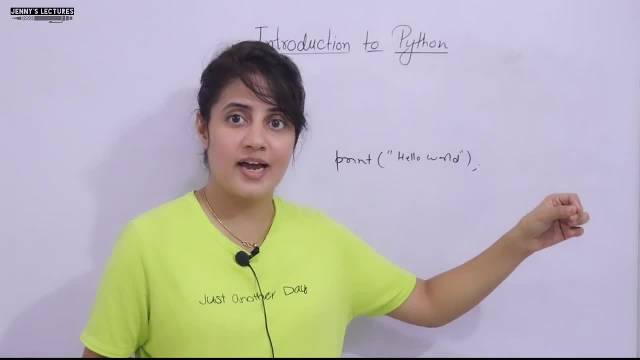 You can reuse that. You don't have to do the whole process from scratch because it will take definitely long time And you don't know- Definitely most of you don't know- how to do that farming process. So same thing, Those inbuilt libraries, packages, modules, functions. 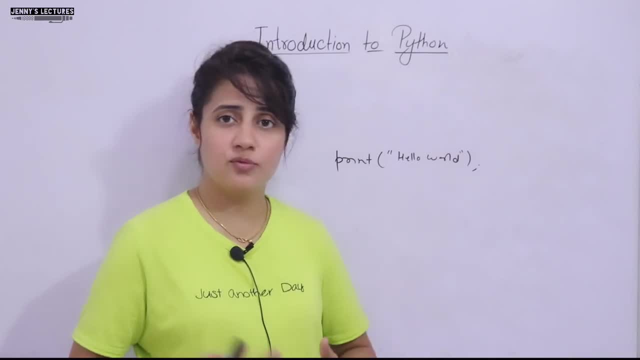 are there. Programmers can reuse those functions, So it saves the time of programmers. And many frameworks are also there, like Django Flask if you are interested in web development. Right, And I told you like automatic memory management is there in this language. 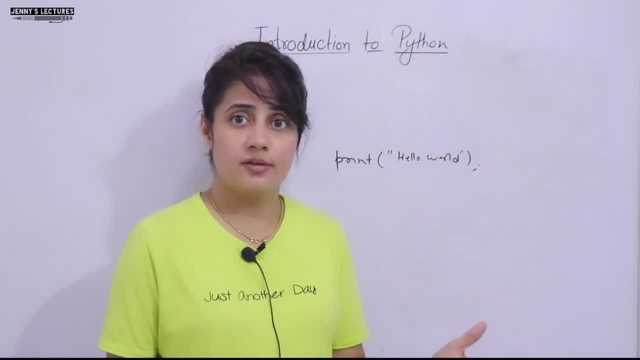 Right, And it is extensible. language You can extend, You can support. More features can be supported, can be added, More libraries or functions can be added. because it is open source, Anyone can contribute in this thing, in this open source code. 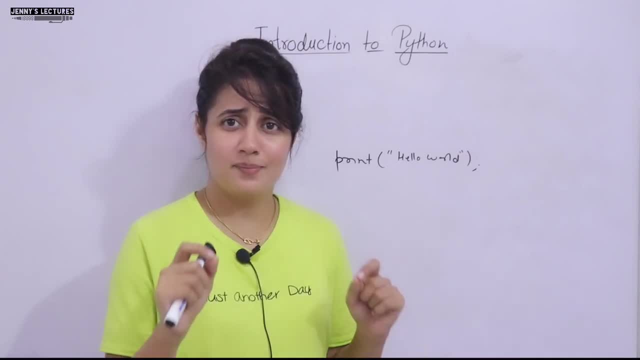 Right, And there are lots of career opportunities also. I'm damn sure this point is very important for you guys. Yeah, There is lots of career opportunities in this field, for this language, Because I told you, this is one of the fastest growing. 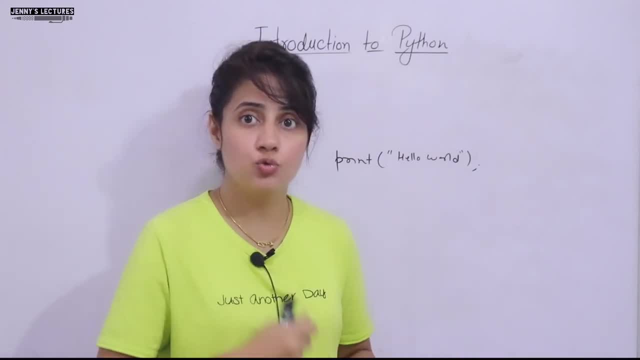 language, in terms of developers, in terms of the companies using this language. Even the big giants like YouTube, Google, Instagram, Google- these companies are also using this language, Python. So there are many career opportunities And average salary is also high. 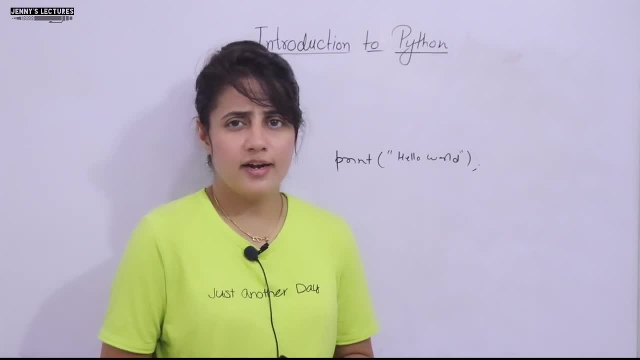 It's from 8 to 12 lakh per annum. So that is why it is so popular And I'm damn sure you are aware about now. this language some features, You are using it, the application areas of Python and all. So please make down your own notes.